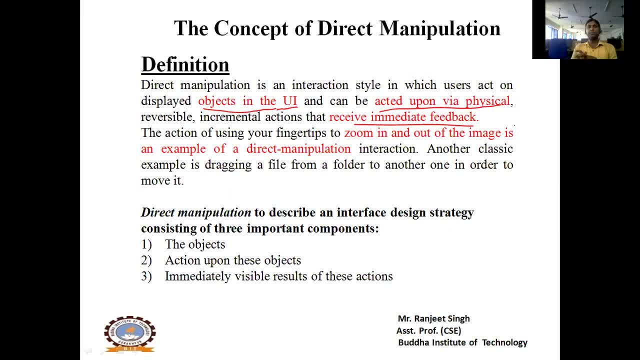 so whatever actions you are performing on that object, you will see a certain feedback and response on the screen. overall, direct manipulation is an interaction where you see lots of objects on user interface or screen on which you perform certain operations, certain actions, and on these actions you receive certain feedbacks. 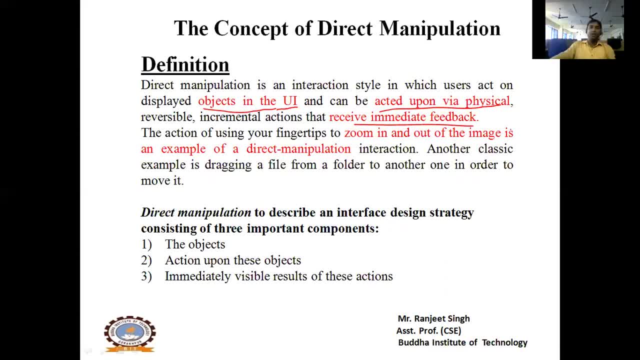 for example, when you zoom in and zoom out any figure, you can do this operation directly. when you zoom in and zoom out any image, this zoom in and zoom out is basically an action. this is an operation, and the image you are seeing on the screen is an object. 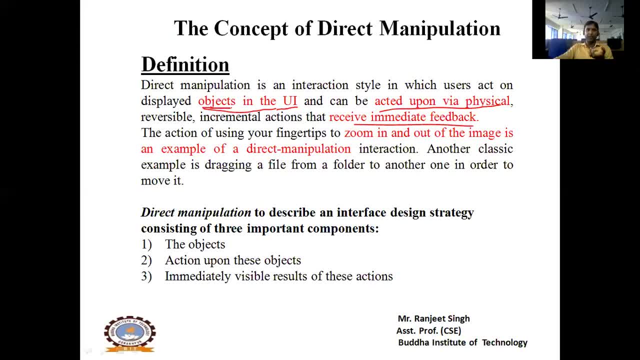 the image you are seeing on the screen. you are performing an action on that object. what is that action? you have to zoom in and zoom out that object. so to zoom in and zoom out that object, you can directly use the system or interface. you can directly zoom in and zoom out that image. 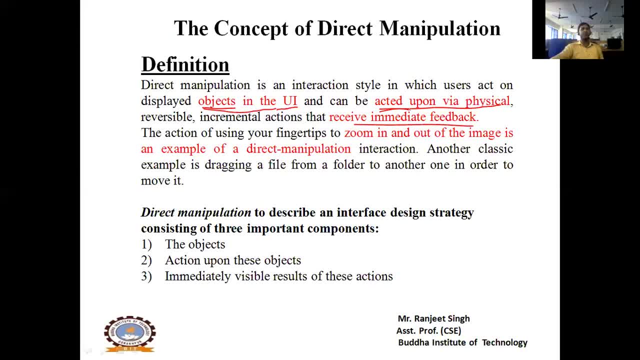 so this overall operation of zoom in and zoom out that image, basically this is what is called direct manipulation, as an example. basically, just like direct manipulation, same way indirect manipulation. so to understand direct manipulation, well we have to understand indirect manipulation, so to clear the difference between direct manipulation and indirect manipulation. 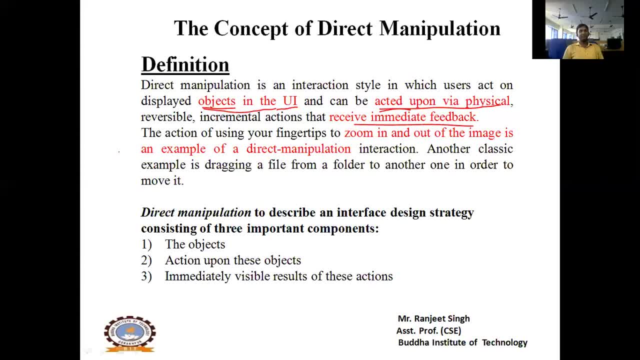 I am taking an example. suppose you have to move any file from D drive to E drive means you have to copy that file from D drive and then take it to F drive and paste it. ok, so you have to copy that file from a certain location and paste it on an observed location. 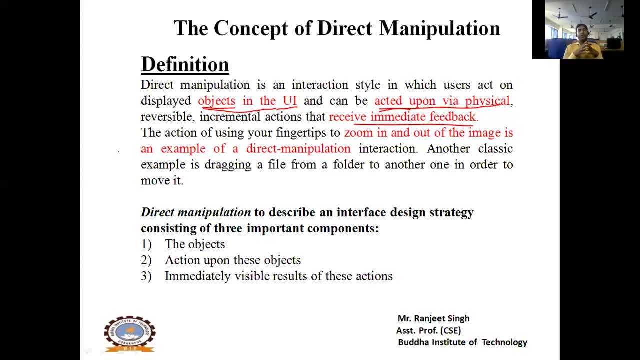 and the operation of moving it. if you do it through command line, then you will have to write many commands through which you have to move that file from one location to another location means to perform that action you are connecting to the system in an indirect way, means the manipulation you are doing. 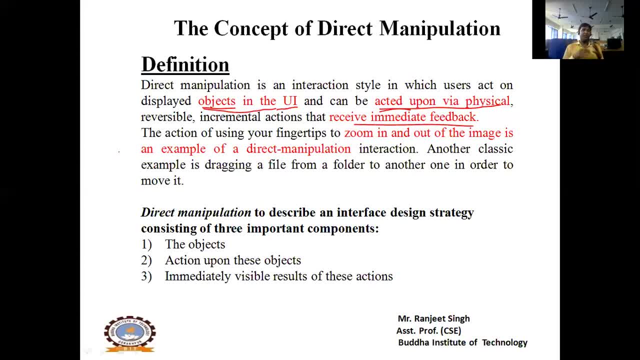 to move the file from one location to another location. that is not direct manipulation. you are writing many commands. after writing those commands, after execution of those commands, then you will perform a certain action. means the action you performed to move the file from one location to another location. 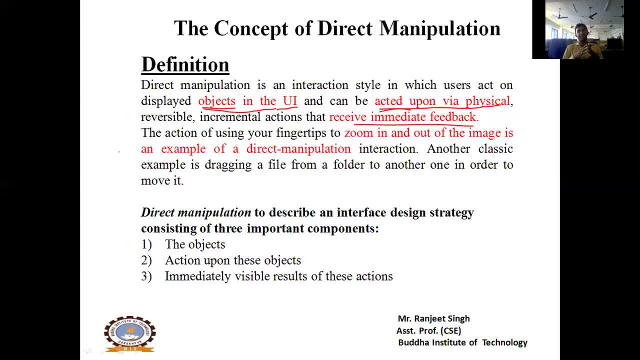 this is not direct manipulation, this is indirect manipulation. but you must have seen, if you want to move any file from D drive to E drive, then you simply drag and drop that file, then also the file will be moved. so we simply drag and drop the file. what we did is: 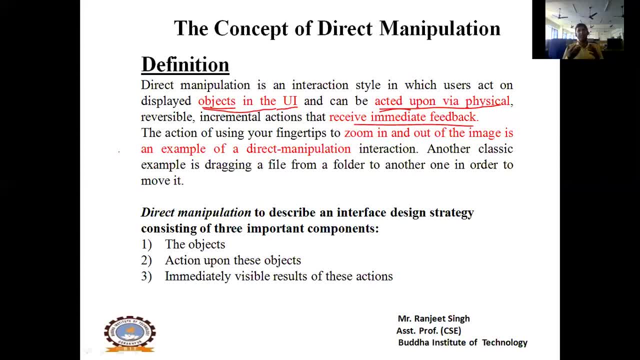 we did direct manipulation, we interacted with the direct system and we simply drag and drop the object or file from the system screen and we moved it and in respect to that movement, we can see a feedback on the screen that a window opens and we can see the file being copied. 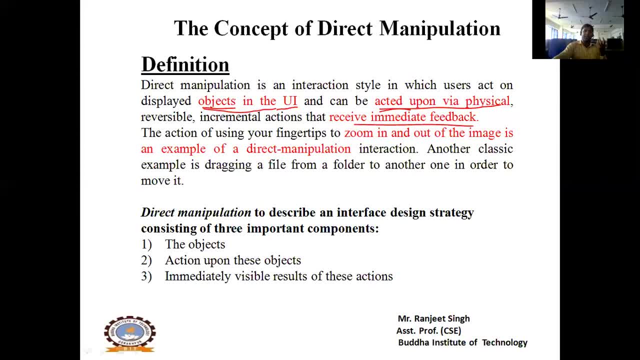 so, basically, the direct manipulation you can understand. direct manipulation is completely based on GUI and indirect manipulation is based on command line interface. you can see it. so if we talk about direct manipulation, then there are three components of direct manipulation, as I told you in the definition. first component is our object. 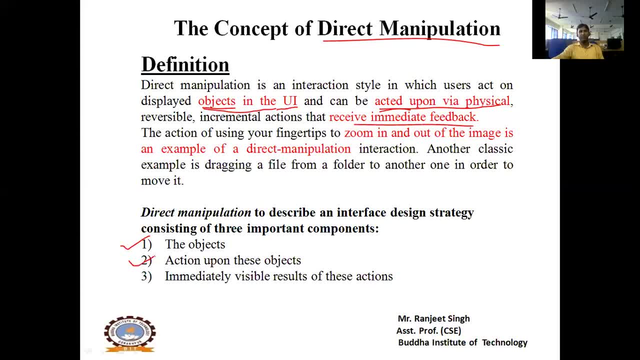 second component is action upon these objects, to perform an action on an object. third component is the result produced in respect to the action you performed. so immediately visible results of these actions means whatever actions you performed, you can see its immediate response, as I told you in the example of indirect manipulation. 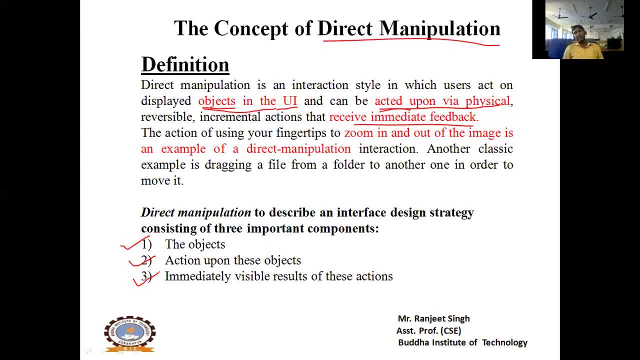 in which you write many commands to move the file. you write commands and the file moves, but you don't see any result in respect to that action. you don't feel on the screen that where my file is being copied. you don't feel anything like that. you don't see any result like that. 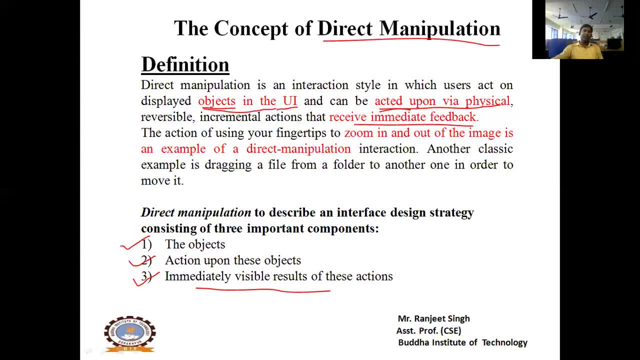 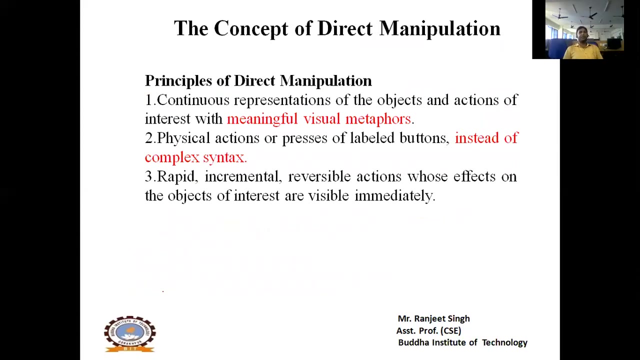 so for direct manipulation these three components are compulsory. it should be of objects, it should be of action, and in respect to that action a result should also be visible. so if we talk about direct manipulation, then these three components are compulsory. in direct manipulation, if we talk about principle, 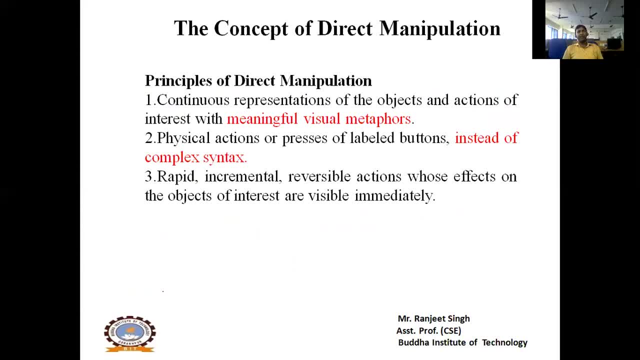 like I told you earlier that you copied a file from D drive to E drive. so basically you copied a file from D drive to E drive by writing many commands. you wrote the command in the machine, you read that command, you executed that command and finally moved the file from D to E. 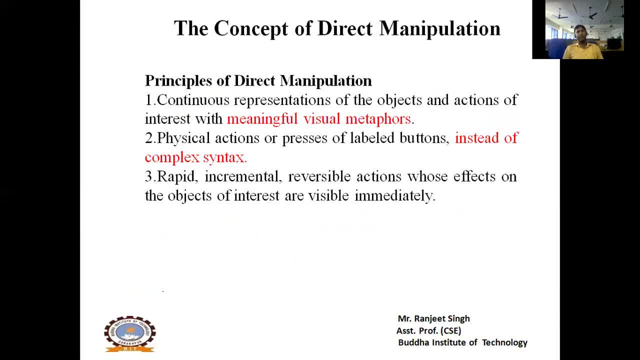 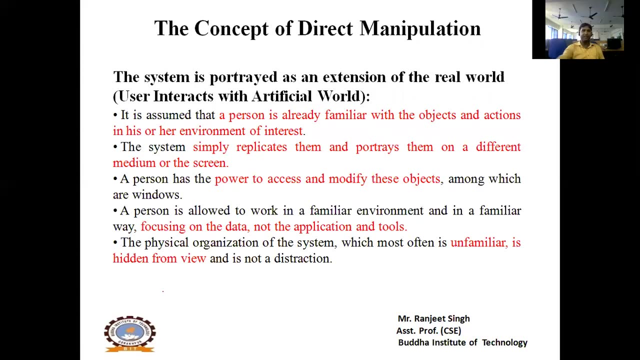 that is real world operation. but when you do direct manipulation, then at that time that manipulation happens in real world environment, not in an artificial environment. as you can see here the system is ported out to as an extension of the real world, means the user interface with artificial world. 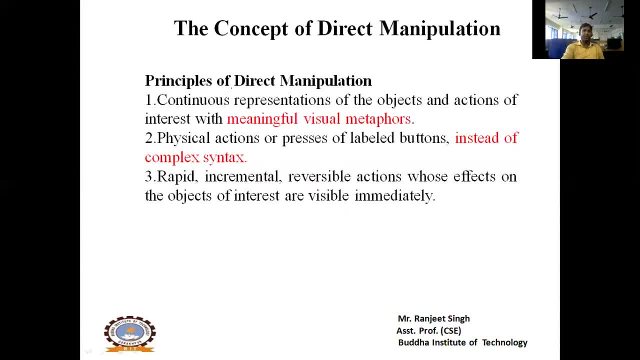 the same work is happening, but in some other way. the same work is happening, system is performing its same operation, but that is happening in direct manipulation. it is happening in such a way that we don't need to write any complex syntax. we can interact with the interface of the directed system. 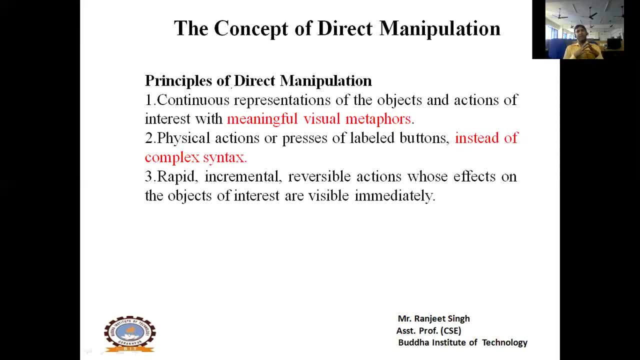 and perform that operation without writing any complex syntax. so let's talk about principle. let's talk about principle of direct manipulation. there are three principles. first one is continuous representation of the object and action of interest with meaningful visual metaphor, means whatever objects which are used in your direct manipulation. 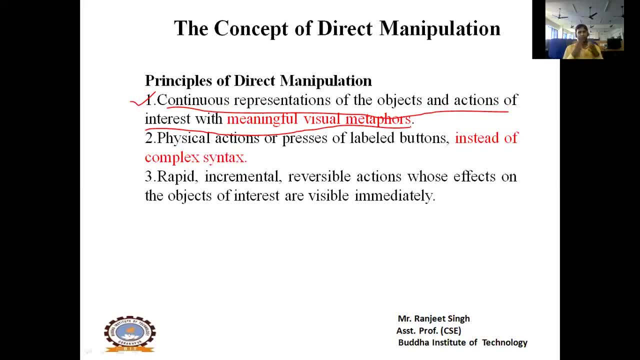 whatever action of interest you have, whatever object or action of interest you have that should be visible to you on your screen. meaning meaning full visual metaphor. means whatever you are seeing on the screen should be displayed this way that you can expect maximum information in minimum time. means whatever object. 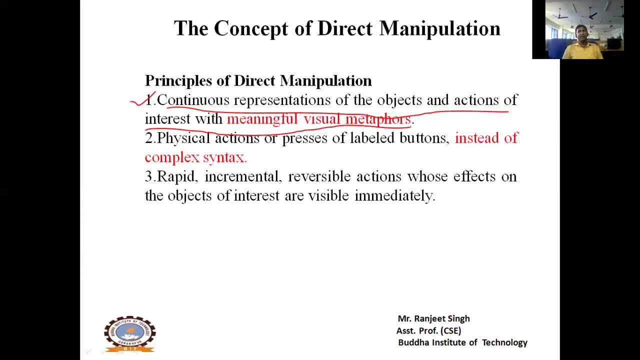 whatever your action of interest is, which you want to use in direct manipulation, it should be in the form of meaningful visual metaphor. okay, so second principle of MRM. second principle is Physical action of faces, of labelled buttons, instead of complex syntax, The action of interest you want to perform on the screen. 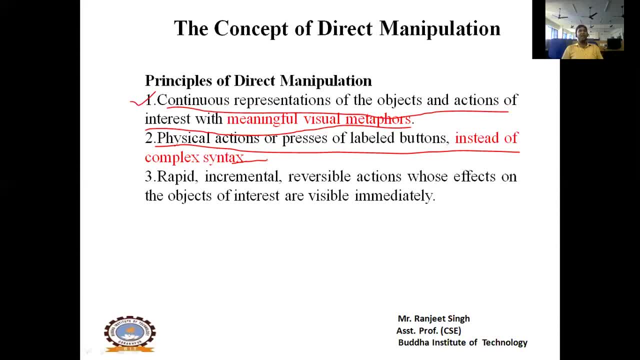 To perform that action you don't need to write lengthy code or complex code. You can perform all those operations using click event or pointing operations. Third principle is Rapid, incremental, reversible action. Those effects on the object of interest are visible immediately. Like I told you about file copying, 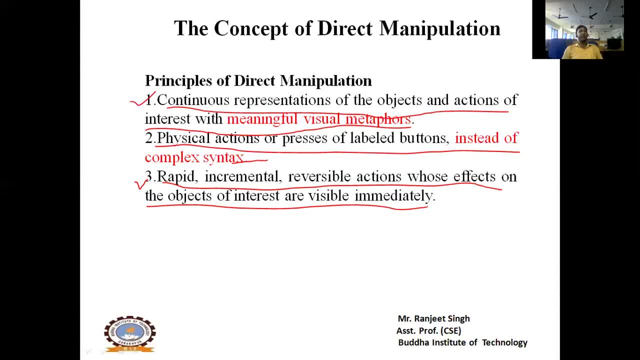 Normally when we copy a direct manipulation file from one drive to another, When we copy and paste it, We feel that our file is being copied from one location to another. location Means there should be visibility In respect of the action we have performed. There should be visibility in respect of that action. 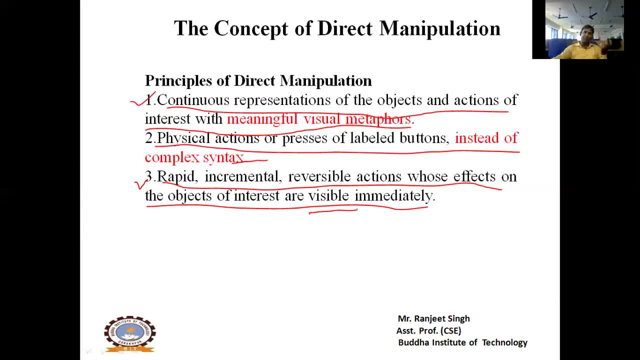 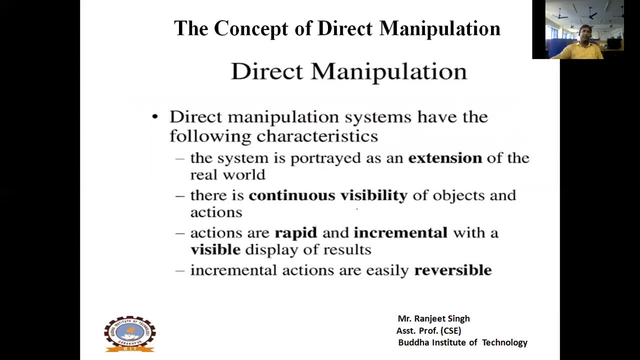 So that we feel that whatever action we have performed on that object, In respect of that action, a response is being produced In direct manipulation. Basically, there are many characteristics. We are talking about 3-4 characteristics here. The first characteristic is: The system is the port yard of an extension of the real world. 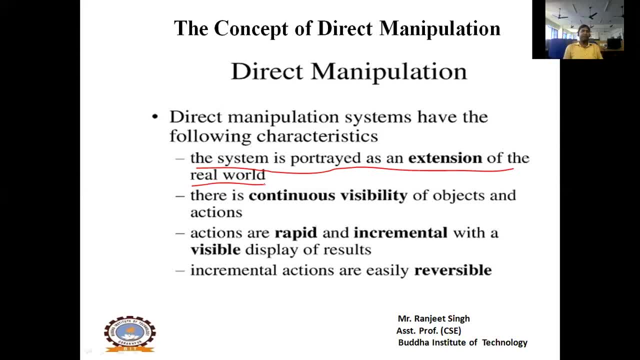 This line means. Let's take the example of file copying. When a file is copied in the real world, There are many commands running internally in the machine. There are many commands running internally in the machine. So the commands running in the machine are the real world. So what we are doing is: 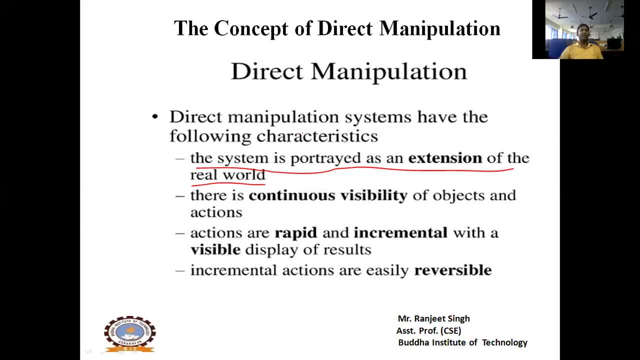 The system is the port yard as an extension of the real world. What is happening in the real world? It will be different from that, But we are doing it different from that By using graphical user interface. So, on the interface, Some certain commands Like this On the buttons or on some icon: 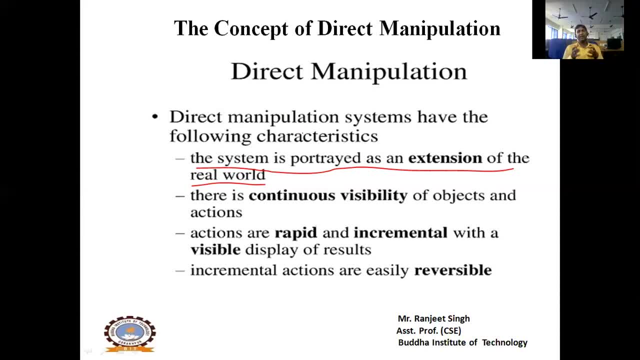 We design and implement it in this way So that we don't see the internal process. We don't know what is the internal process, But we can see the response of that action on our screen. So that is called direct manipulation. The system is the port yard as an extension of the real world. 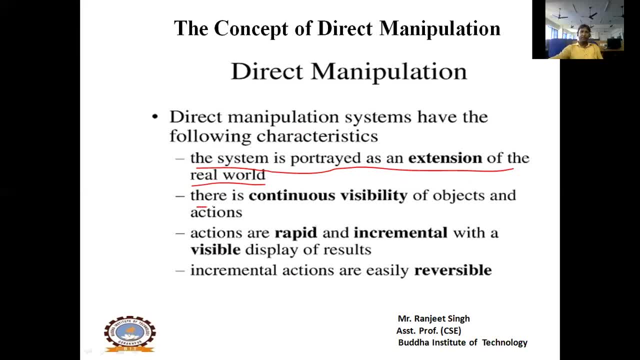 Next is There is continuous visibility of object and action, Whatever the object on which you have to do the operation. I have talked about copying the file, So the file is an object here. Now, whatever action you are going to perform on that file Means you are going to copy. 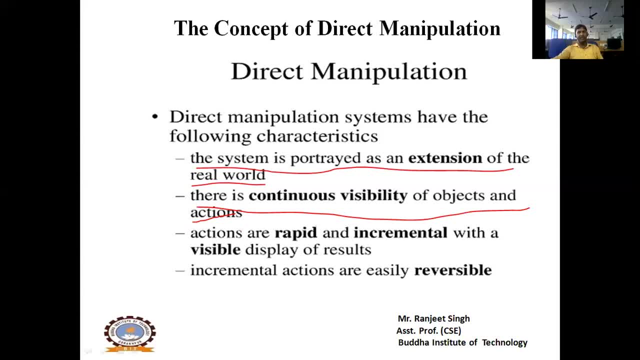 So as soon as you right click on that file, So you see many options. There is a copy option in this, So the action you are going to perform, It should be visible. Next is: Actions are ready, Rapid and incremental, with a visual display of result Means if you have performed the proper test. cooperation. 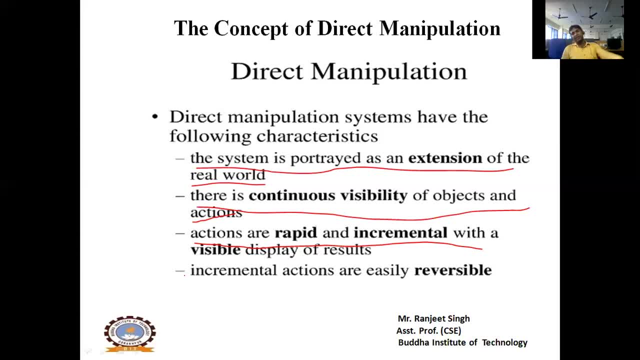 Regarding that on your screen There should be some display, There should be something visible Through which you feel that you have performed the action. It is being executed properly. Incremental actions are easily reversible, So overall it means That on your screen, Whatever the objects are, Whatever the operation you are performing on those objects, 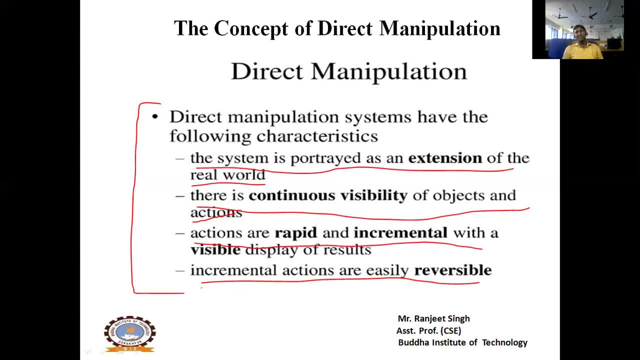 Whatever the reaction of those operations. All of these things, All of these things Should be visible. We should see the object We are going to perform the action. It should be available as an option on the screen And after performing that action, Its execution should be visible on the screen. 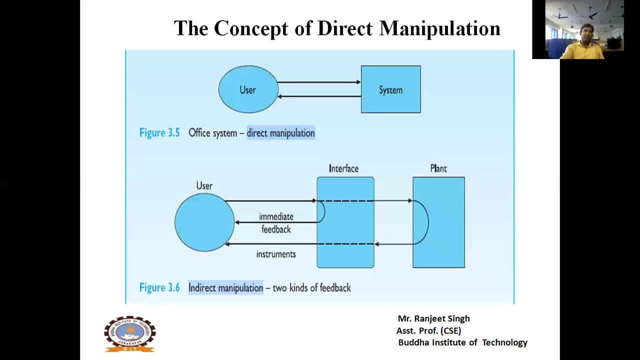 What is being performed Right. So you see here Direct manipulation and indirect manipulation, Which has been told here. User directly interacts with the system And performs a certain action. Okay, Now, what is that action? We don't care about that And the system performs that action, A certain response. 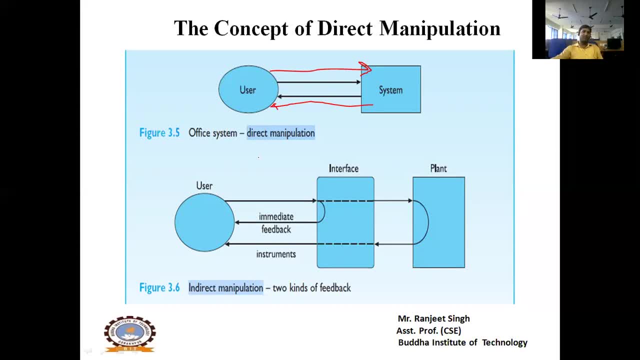 Or you can say: Result is produced. Okay, This is a direct manipulation, Like, Let's say, I am driving a car And I saw from the car window That There is a big pit in front of the road. So what I will automatically do? I will turn the steering wheel of my car. 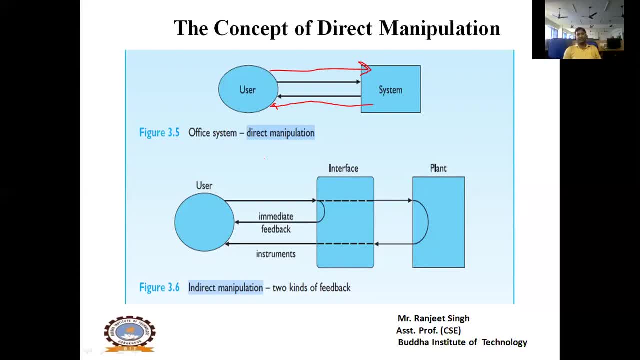 And turn the car in such a way So that my car doesn't go into the pit. So what I did was direct manipulation. I saw the objects, Saw the pit And I tried to perform a certain action: That I turn my car So to perform that action. I did direct manipulation. 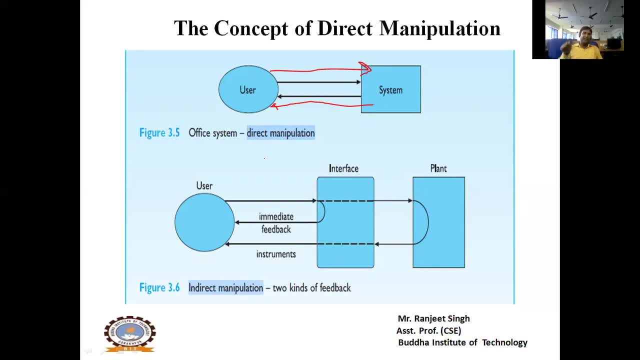 By using steering of the car. I performed the steering of the car So because of that manipulation The car got diverted. So this was. direct manipulation Means To perform a certain action. When we perform a certain action directly For that object, We feel the result. This is called direct manipulation. 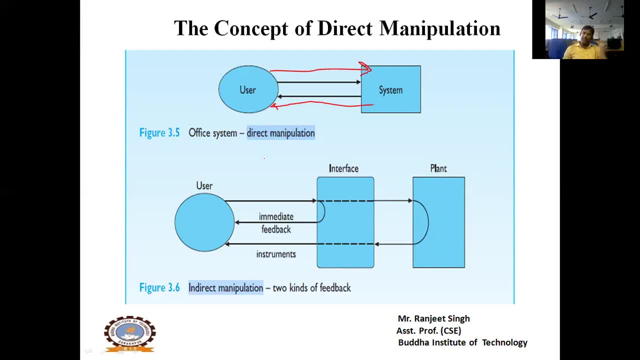 Okay. But if we talk about indirect manipulation, As you can see in the figure, There is a user, There is a plant- Okay, And there is an interface. So this user, If he wants to perform a certain action on this plant, Okay, So he can't perform a certain action directly on this plant. 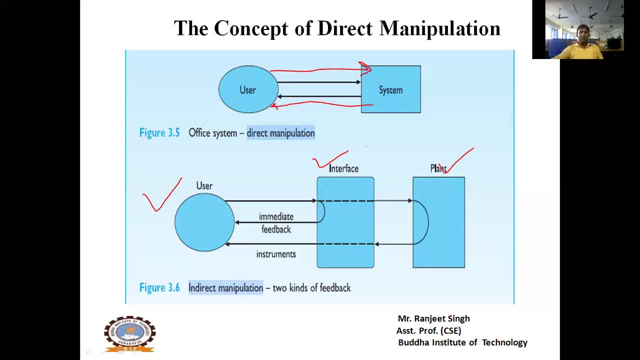 Okay, He will write certain commands through this interface. Graphically There is no interface. You understand this. This is a command line interface. He will run certain commands through this interface. Those certain commands will go to the plant. There will be an execution on the plant. After execution he will give a certain response. 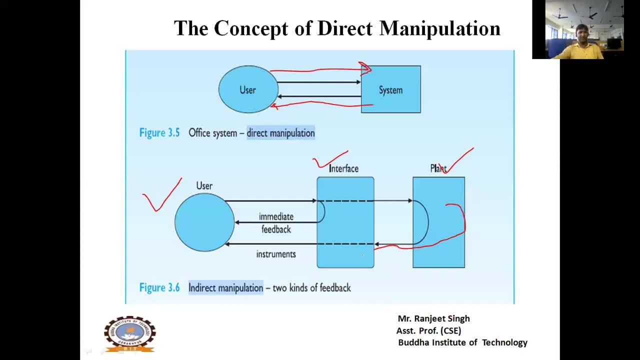 Then, on this interface, A certain result will be produced Which this user will read And identify. What response did the system give? So what I mean to say is: This user Is not able to directly interact with this plant. He is interacting through this interface, And this interface is such an interface. 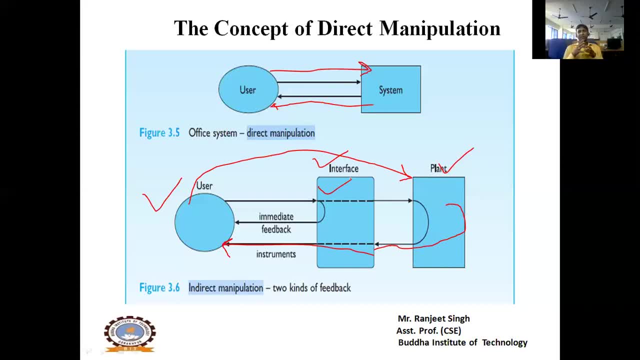 Which is not allowing the action to be shown. Neither You are Being able to see the objects properly, Nor The result that you are getting. That result is in this form: That To understand it, To read it, To extract the information from it, You need to be a skilled person. 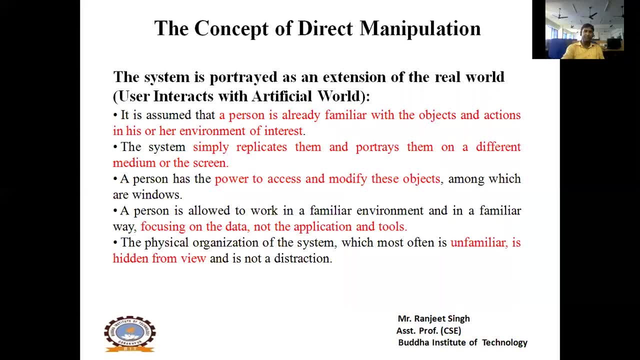 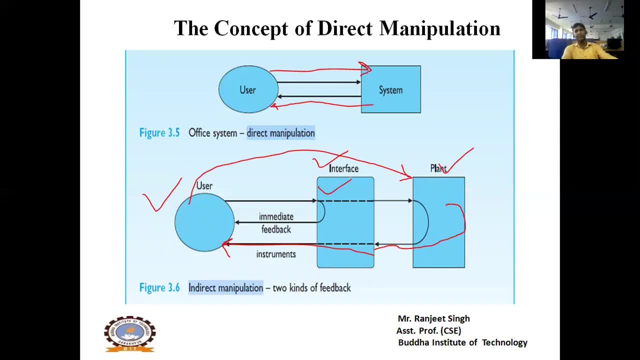 On that domain. Okay, So The direct manipulation. I just showed you the difference between direct manipulation and indirect manipulation By using figure. So, Through this example, I told you earlier That this file is copied Through DOS, Through command line, Through command line. So that is indirect manipulation. But if we do it through an interface? 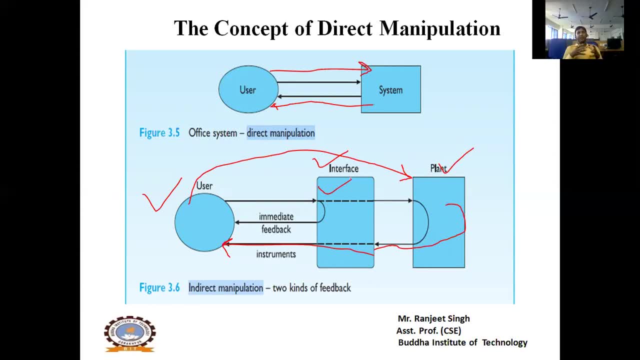 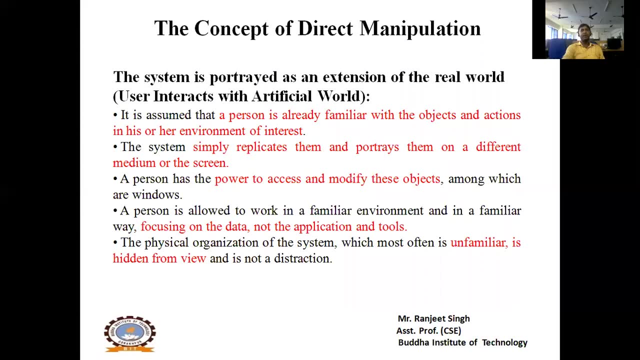 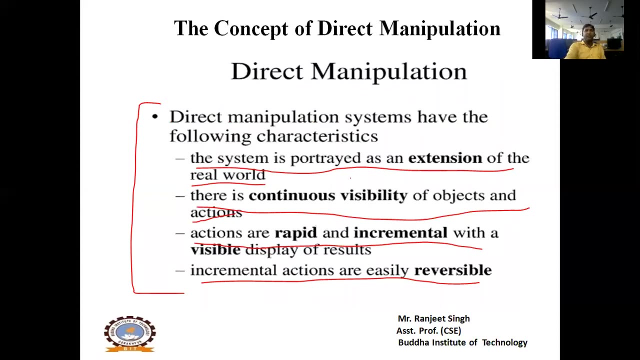 Or if we do it directly on Windows. So what is that? That is our direct manipulation. So these are the differences between direct manipulation and indirect manipulation. We will talk about it further. Now, What You Have, These certain characteristics, You have seen these characteristics: The system is portrayed as an extension of the real world. 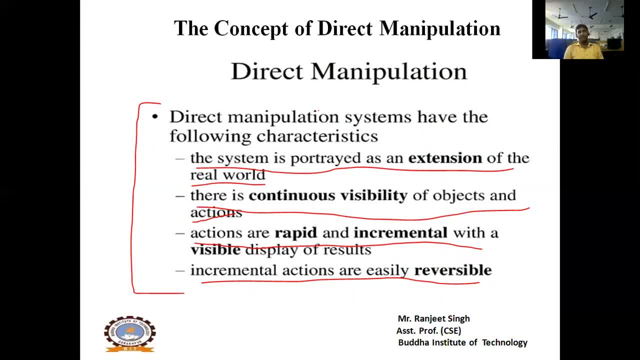 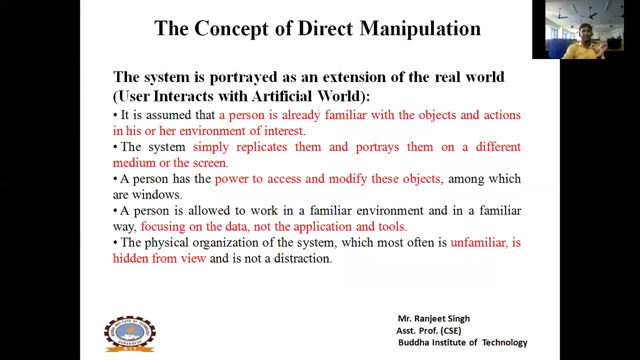 There is continuous visibility of object and action. Action are rapid and incremental, with the visible display of results Means whatever object is seen, The action that is going to be performed should also be seen And the result should also be seen. All these are our characteristics. These characteristics, We will understand them one by one. 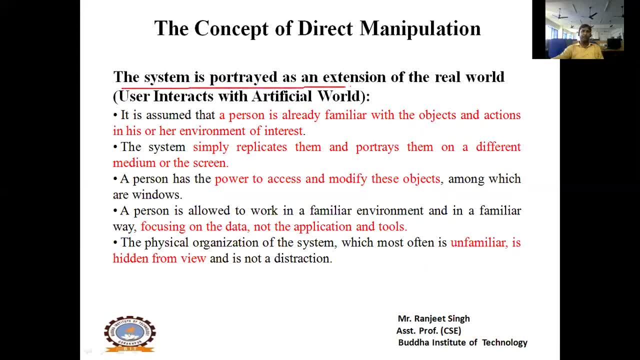 As it says here, The system is portrayed as an extension of the real world. What is happening in the real world? That same thing. We have to represent it in a graphical form in some other way. So the other way is: What is that Our artificial world Means? What is happening in the real world? 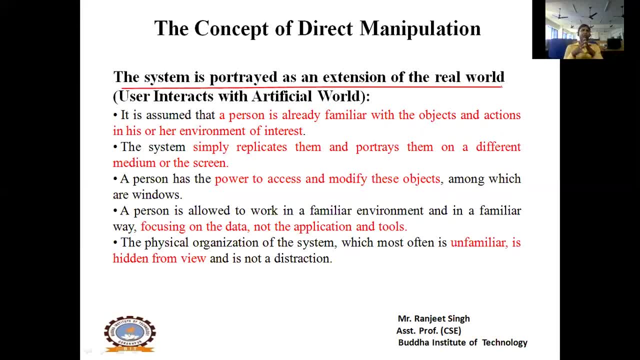 What is not happening, We don't know, But we are feeling those things. We are feeling those things. Means: There There is visibility of object, There is visibility of action And There is visibility of results. Means: It is assumed that A person is already familiar with the objects and action. 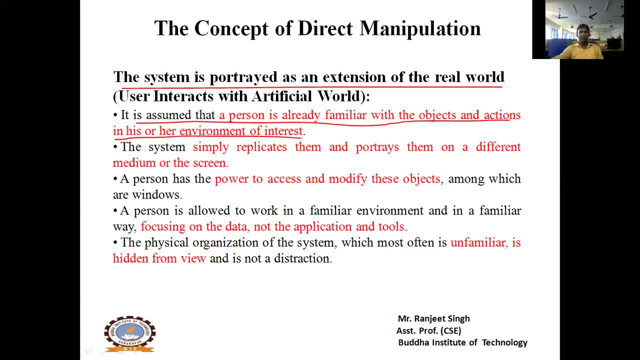 In his or her environment of interest. Whatever the user is, He is familiar with all the objects of his environment Aware. The system simply replicates them And portrays them On a different medium or the screen. Whatever the operations are, All the information of the operations Should be properly generated on the screen. 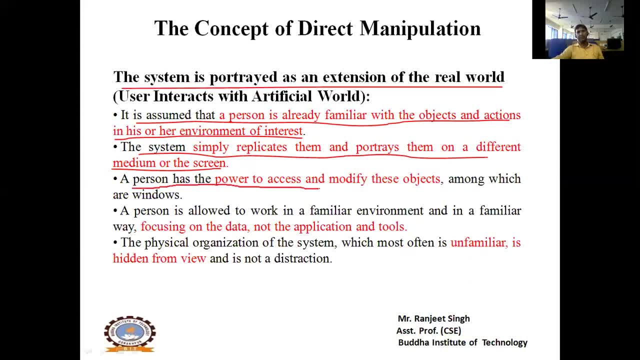 The person has the power to access and modify these objects, Among which Are windows. Whatever is being displayed on our screen, We can directly manipulate it. A person is allowed to work in a familiar environment, In a familiar environment And in a familiar way, Focusing on the data. 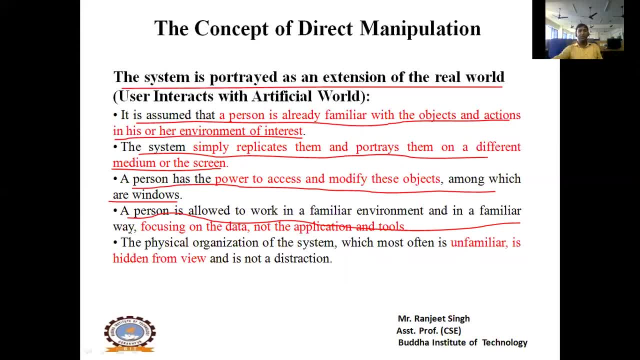 Not the application tool: Focusing on the data, Not the application tool. A person is allowed to work In a familiar environment, On the graphical environment Or on the direct manipulation environment. We are working For that environment, We are familiar with that environment. It should be clear. We should focus on the data that we are using. 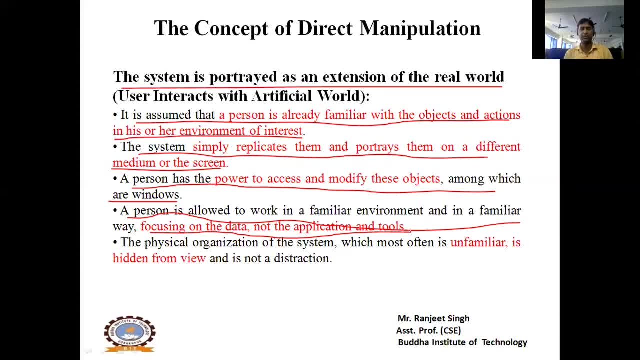 This does not mean That which application, Which tool should be used. For example, Like I told you earlier, I am driving a car, I am on the road, My car is not working, So I turned the steering wheel of the car And diverted the car's route- Basically what I have done in this. 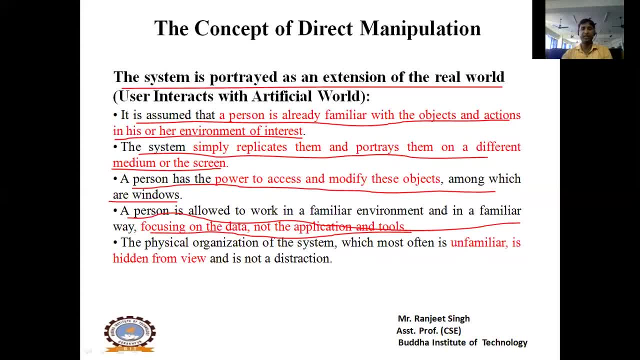 I focused on the data. Focusing on the data, I said focusing on the data means I have seen a pit. I don't want to go into the pit. this is my data. I have to focus on this. for that, I have diverted the steering wheel from the car. 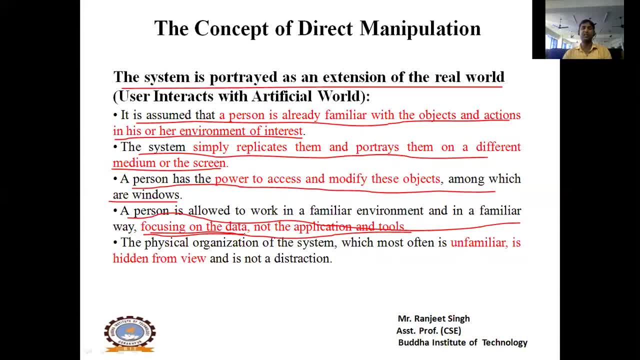 now, how the steering wheel is moving, how the internal gears are working, I don't care, I just have to divert the steering wheel from the car. the physical organization of the system, which most often is unfamiliar, is hidden from the view: all the information of the system, all the aspects which we are not familiar with. 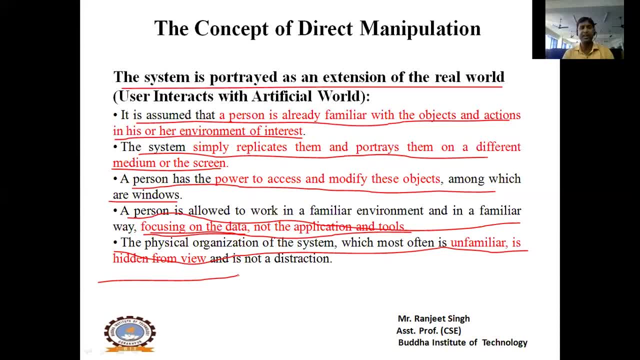 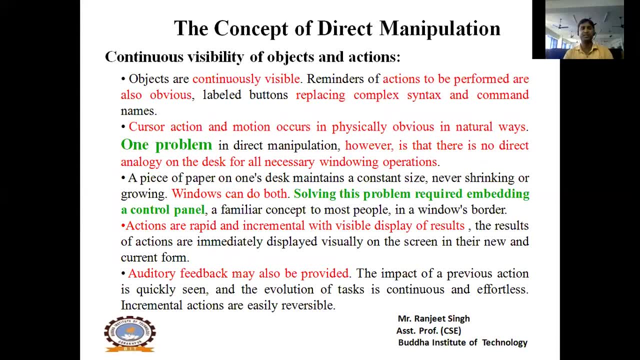 we have to hide them, we don't have to show them. next is continuous visibility of object and action. same thing is coming again and again: we have to see the action, we have to see the object and we have to see the result. so the continuous visibility of object and action means whatever operation you are performing, 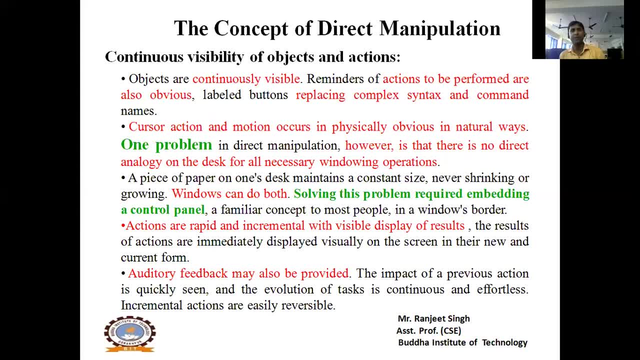 ok, so the object should be visible before the operation is performed and after the operation is performed. and after the operation is performed, the action should be visible in the middle slot means objects are continuously visible. reminder of action to be performed are also obvious. ok, means objects should be visible and actions to be performed are also obvious. 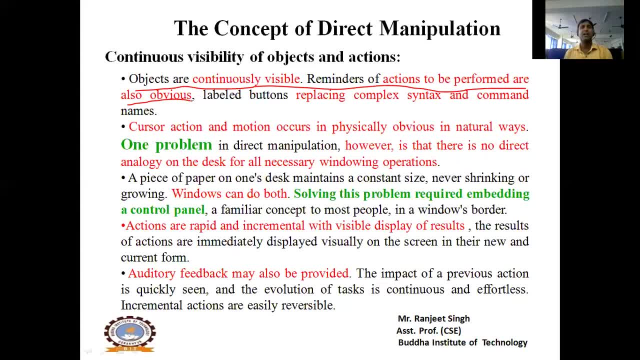 the action which is being performed should also be visible. labelled buttons replace complex syntax, and commands means the commands which we used to write in CMD, the commands through which we used to do indirect manipulation without doing that indirect manipulation, without writing commands. what should we do? 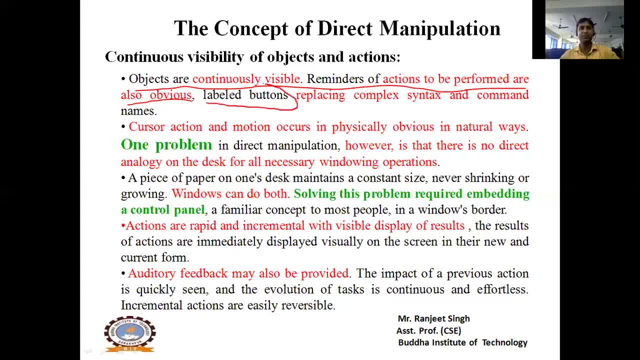 we should use labelled buttons. we should use labelled buttons so that we can see the labels on the buttons, so that we can see which operation or which action should be performed with this button means objects should be visible and the certain operation which has to be performed on that object. 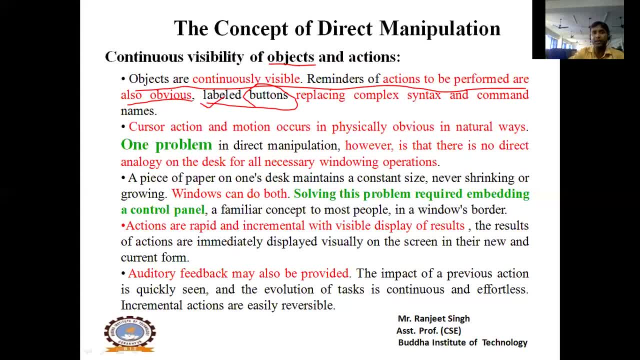 regarding that operation. we have to do proper levelling on the button, like if you right click, then in the list which is displayed there is a copy option, refresh option. all those buttons have certain click events performed on them and we do levelling on them so that we can understand. 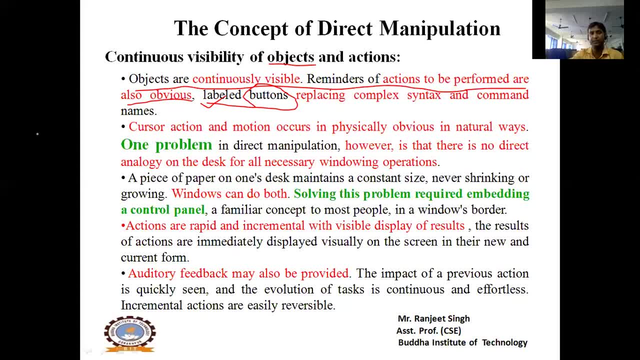 which action will be performed with this button. cursor action and motion occurs in physically obvious, in natural way. normally, whatever action we do is done by pointing devices. cursor action occurs. one problem in direct manipulation- how it works- is that there is no direct analogy on the desk for all necessary windowing operation. 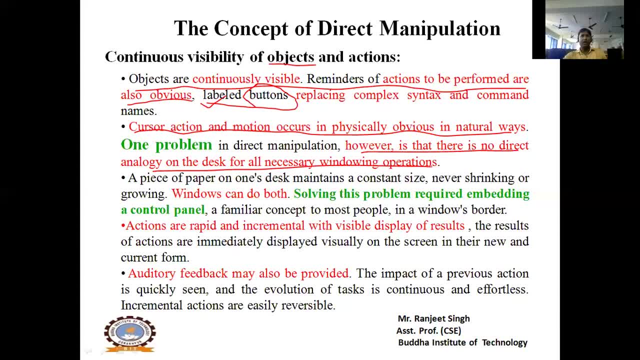 it is not necessary that there is direct analogy for every window operation. that is why in direct we do direct analogy on every object. we cannot perform direct manipulation on any object. that is why we have to perform indirect manipulation on certain objects. ok, if piece of paper on one desk maintain a constant size, never sink or go in, windows can do both. 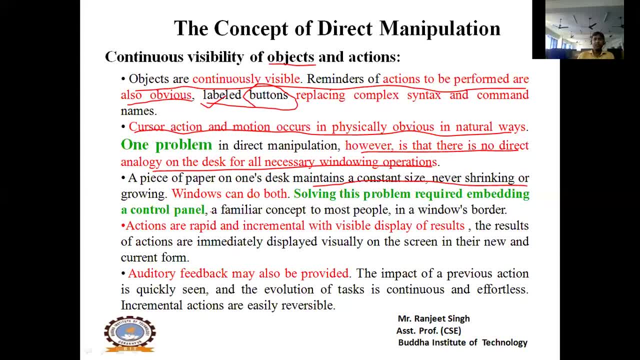 this is what he is trying to say. suppose you have written something on the paper. you have written a lot of sentences. you cannot change the font size or font style in that sentence. but when you write the same thing on any system or word processing software, then you can directly manipulate it. 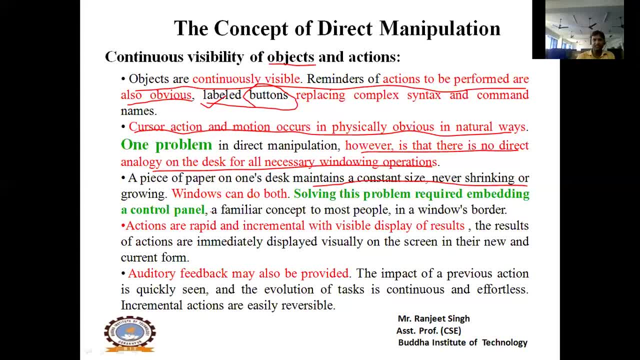 you can increase its size, you can change its font style. you can change the font size. you can perform all these changes directly on it. actions are rapid and incremental, with visible display of figures. whatever action you are performing, its result should be visible on your screen. auditory feedback may also be provided. 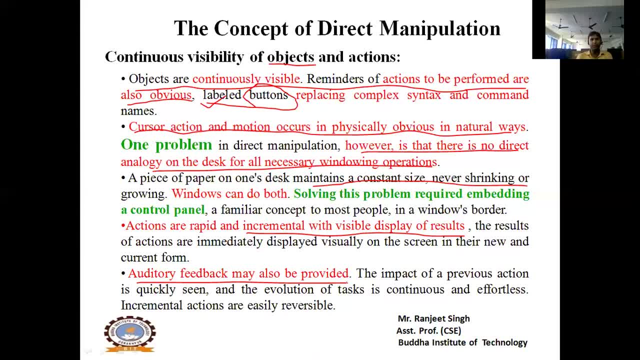 feedback may also be provided in the form of audio. overall, it means that visibility is very important in direct manipulation, whether it is the visibility of object, whether it is the visibility of action, like we have done leveling on buttons- it represents the visibility of action and the result that is being produced in respect of that action. 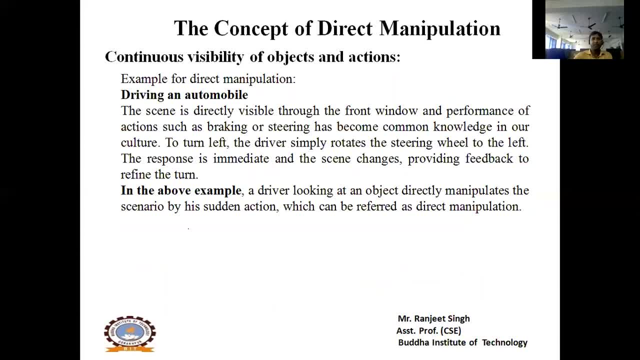 that is the visibility of that action. next is continuous visibility of object and action. earlier I told you an example of driving a car. so how is the direct manipulation happening in this? by steering of the car. by using the steering of the car, what we are doing directly? 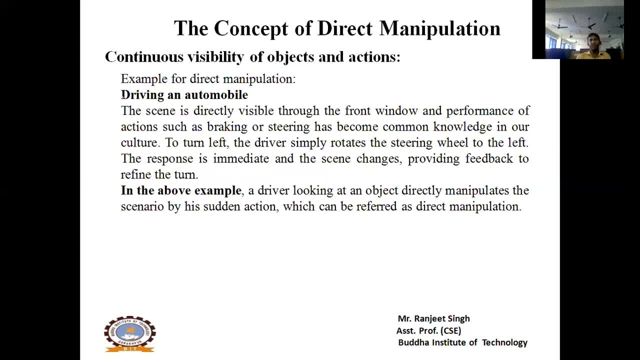 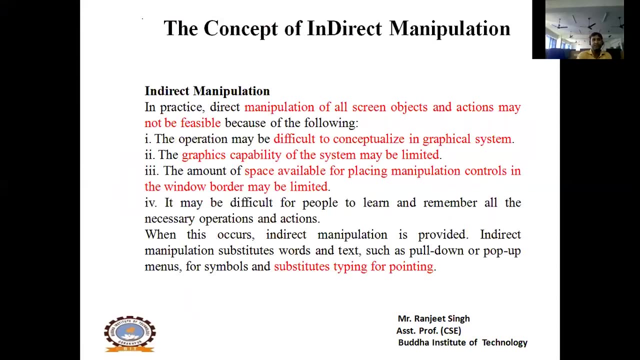 we are able to perform a certain action or manipulation on that object. so this was your, basically this section. this is your example, which represents the direct manipulation, how it is really performed. now we will talk about direct manipulation. in practice, direct manipulation of all screen objects and action may not be feasible. 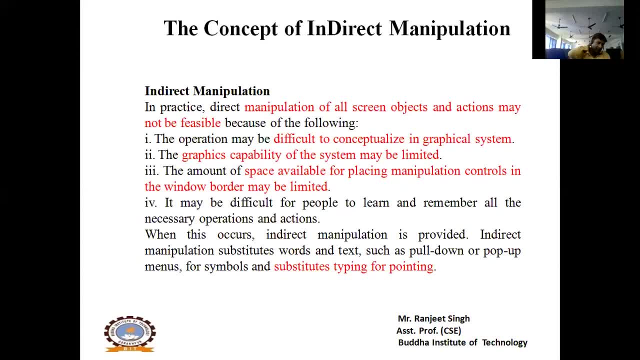 like earlier, I told you that there are many screen objects, but we cannot perform direct manipulation on every screen object. so we cannot perform direct manipulation on such screen objects. on that, we cannot perform direct manipulation on such screen objects. so now we will look at certain points and we will know. 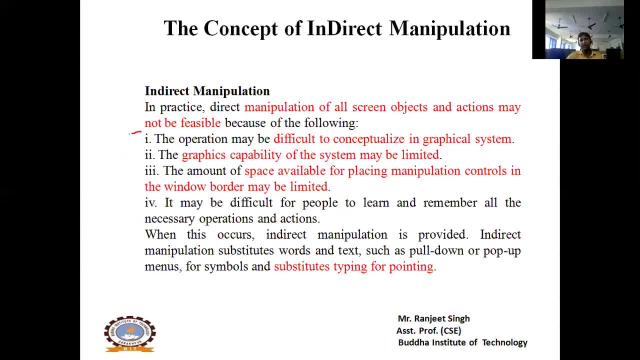 that why we cannot perform direct manipulation on certain objects. the first reason is given here: the operation may be difficult to conceptualize in graphical system means your concept which you want to implement on direct manipulation or on which you want to perform direct manipulation, we cannot get it in graphical system. 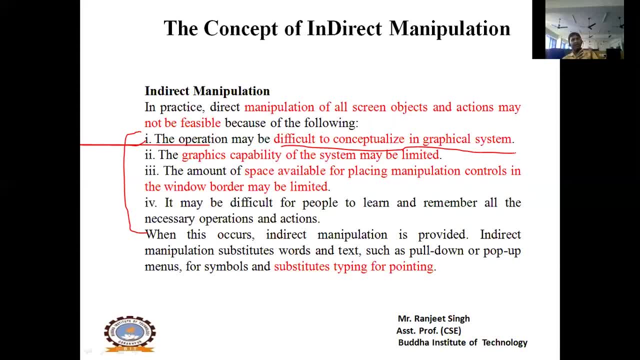 we cannot convert it in graphical system, so we perform direct manipulation on it. in next IC the graphic capability of the screen object may be less than the graphic capability of the system may be less than the graphic capability of the system. because of this we cannot perform direct manipulation on that object. 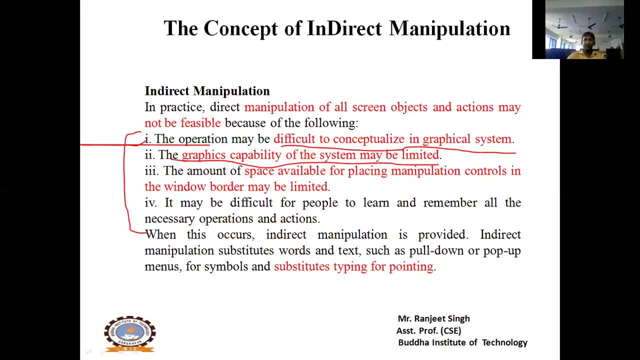 like batch file processing. normally you have to execute many files at once. so what you do is you make collection of many files and you provide all those files to CPU. CPU will execute them one by one. so all these processes which we execute in direct manipulation, the amount of space available for placing manipulating control. 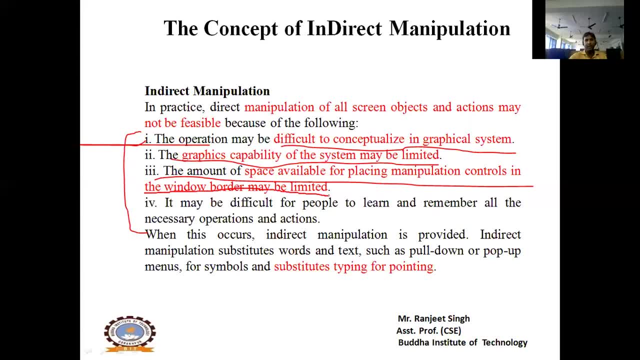 in the window border may be limited, for example, the size of the screen. you may not be able to fit that object or the control system you want to design for. that may not fit in the screen border. it may be difficult for people to learn and remember all the necessary action and operation. 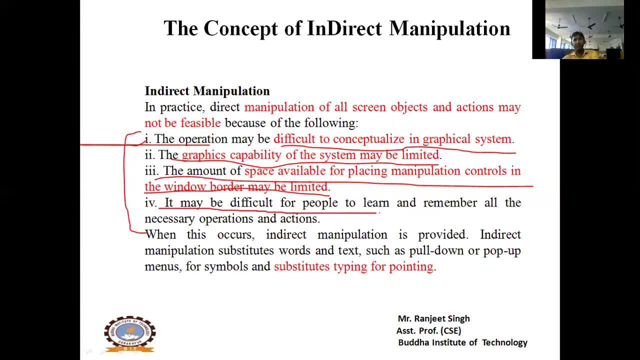 this one. it may be difficult for people to learn and remember all the necessary operation and action. while this occurs in direct manipulation is provided so many such operations and actions which human beings cannot learn easily, nor can they use it easily. so there are many such drawbacks, due to which. 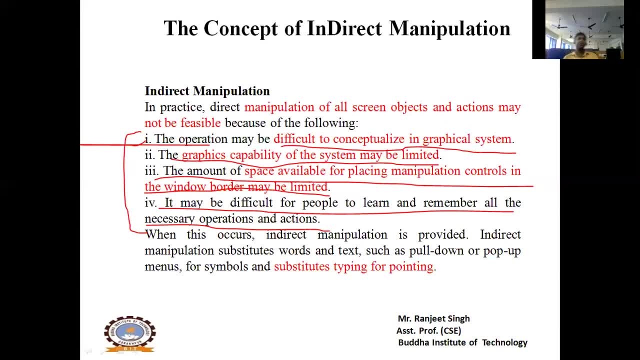 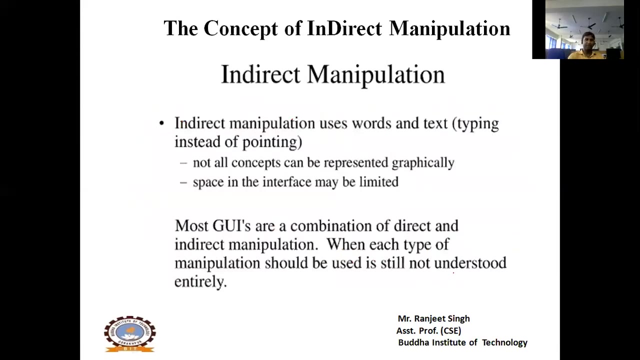 we use indirect manipulation and basically indirect manipulation substitutes typing by using pointing. overall it means in short, you can understand that the direct manipulation is based on GUI, the indirect manipulation is based on command line. indirect manipulation uses word and text, as I told you earlier that they are based on command line. 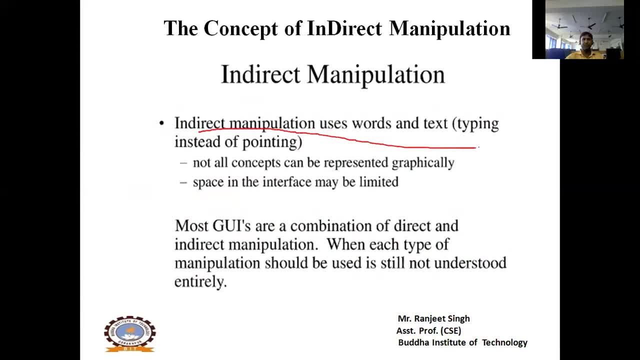 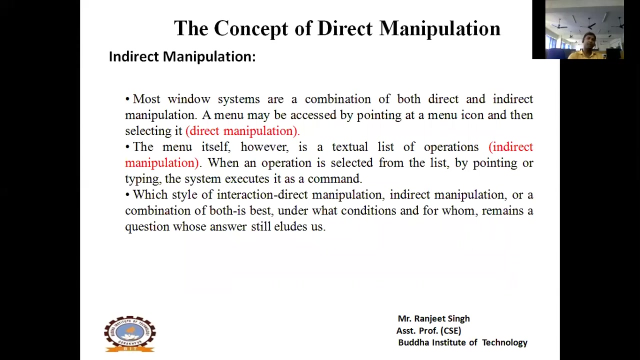 indirect manipulation uses words and text instead of pointing. not all concepts can be represented graphically. space in the interface may be limited. but one more thing: there are many examples in the interface in which we, along with direct manipulation, also use indirect manipulation. ok, for indirect manipulation, see here. 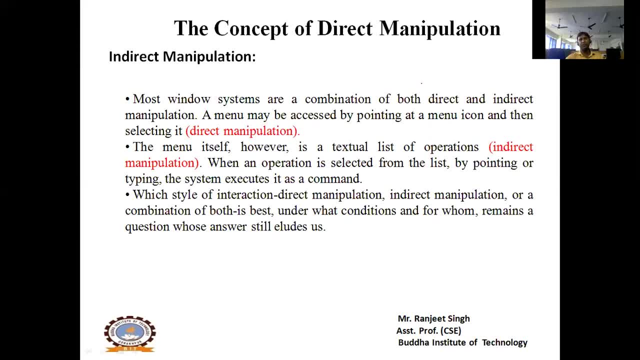 most window system are a combination of both direct and indirect manipulation. a menu may be accessed by pointing at a menu icon and then selected it. direct manipulation means clicking on any menu and selecting any option is a kind of direct manipulation. the menu itself, however, is a textual list of operations. 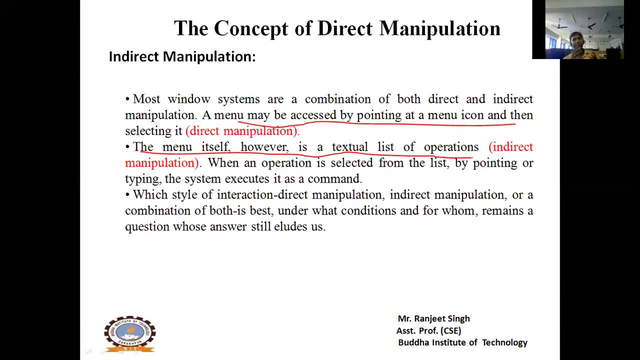 indirect manipulation. but basically, what is a menu if we see internally, then on every option of the menu we have defined many actions. so the actions performed internally, what is indirect manipulation? the menu itself, however, is a textual list of operations. ok, in that we have defined all the commands. 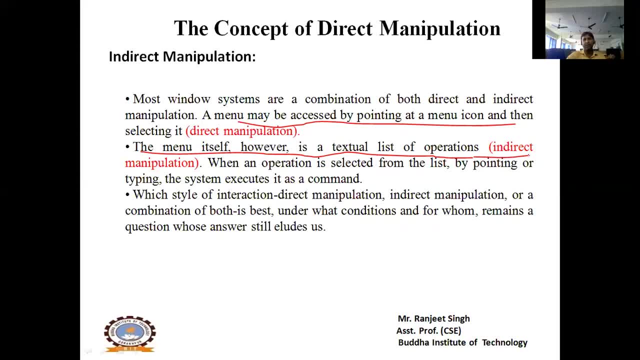 on that menu and as we perform a click, certain action is executed and direct manipulation is performed. but behind that direct manipulation means a textual list of operations. ok, I could say indirect manipulation: when an operation is selected from the list by pointing and typing the system, execute its. 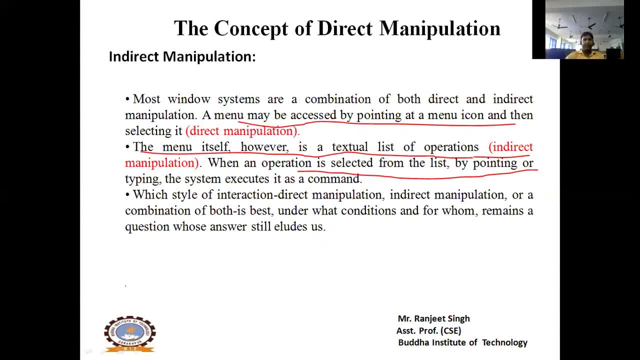 as a command. which style of interaction- direct manipulation, indirect manipulation or a combination of both- is best, under what conditions and for whom, remains a question whose answer is still in looses. overall conclusion here is that direct manipulation is such a manipulation in which visibility is very important. 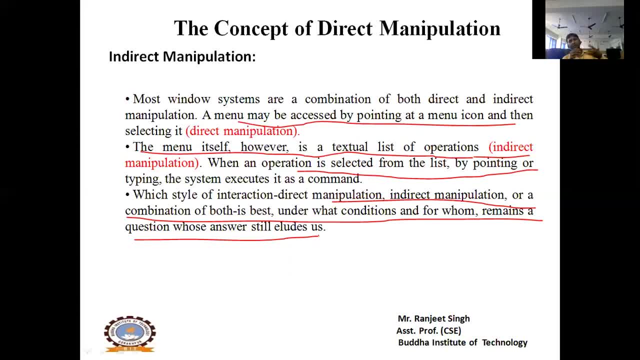 and that visibility should be on those three entities on which objects on action and result on objects. on objects means we represent it in the form of icons or in some graphical form. on action means we use some label on those buttons so that we know which operation is to be performed. 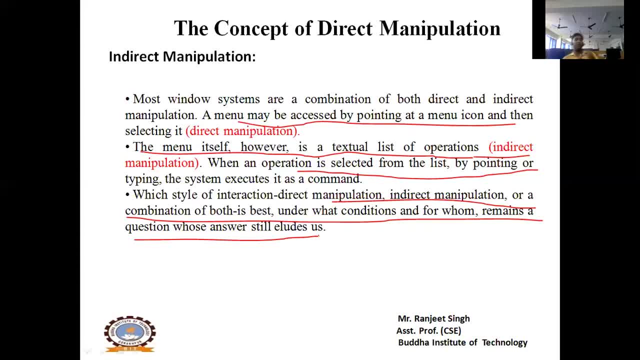 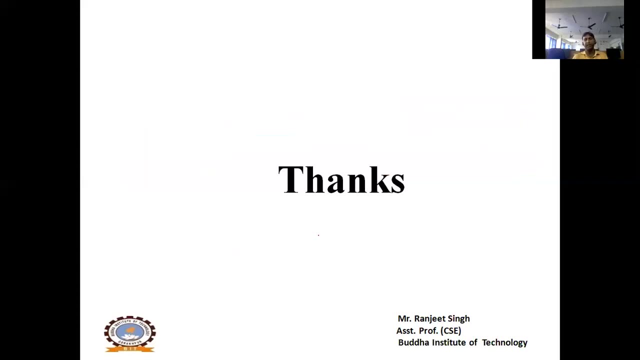 results, like whatever action is being performed, whatever result is being produced, we represent it graphically so that user gets a feedback that certain operation is being executed. so i think direct manipulation or direct indirect manipulation concept you must have understood. thank you.